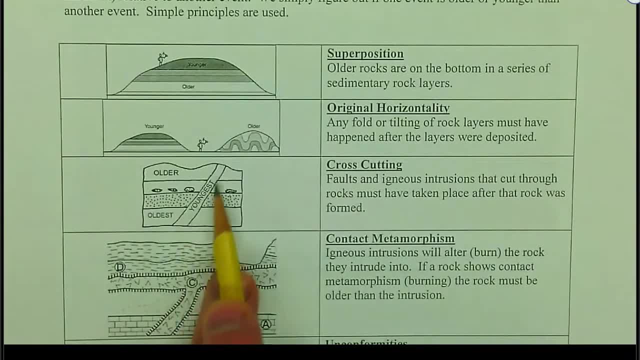 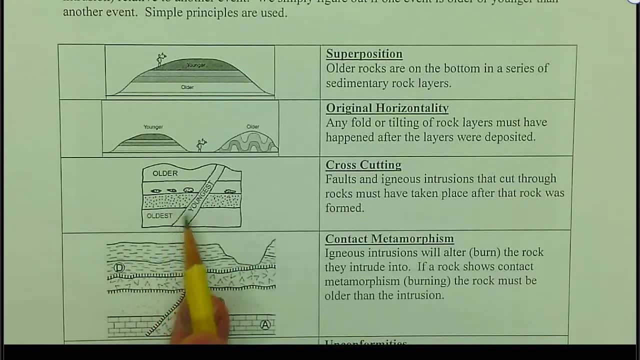 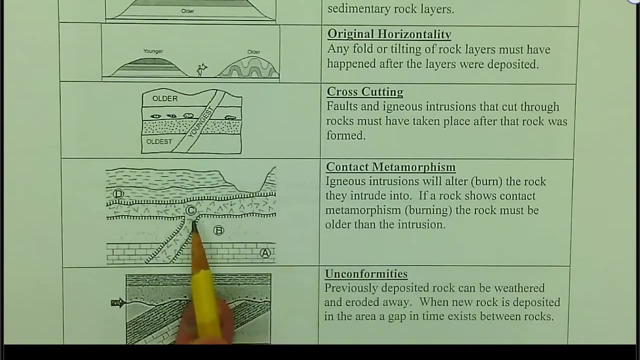 have happened after the rocks were there. The same thing is true about igneous intrusions and faults. Any rock that gets intruded or faulted, the rock must be older than the intrusion or the fault. We talked about contact metamorphism When a lava or magma touches a rock. 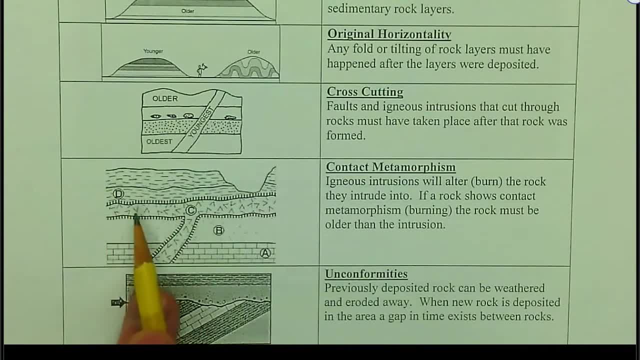 it's going to create a zone of contact metamorphism. We usually show that with these little tick marks. The rock has to be there in order to get burnt or have contact metamorphism. Anytime we see contact metamorphism, we know the rock that has contact metamorphism. 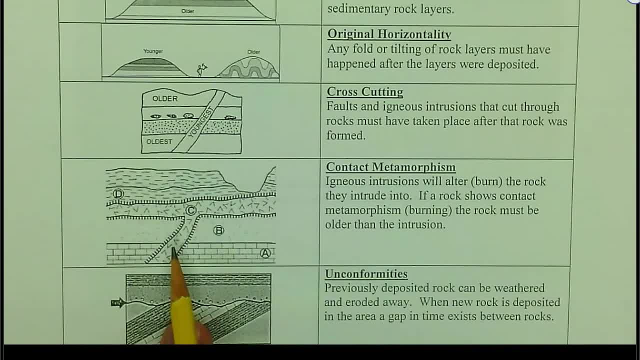 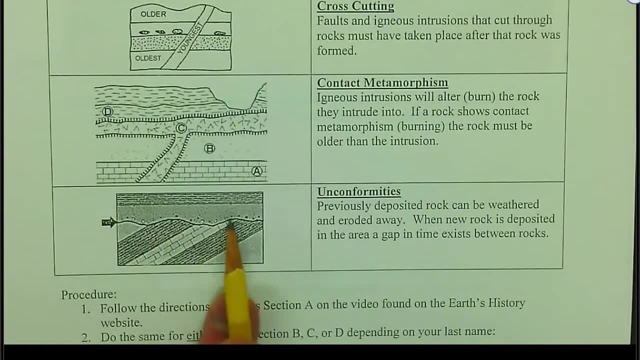 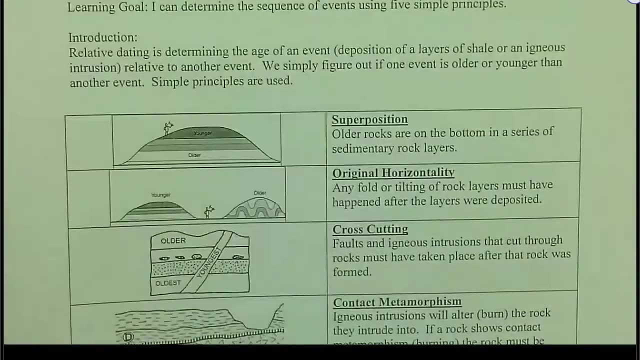 must be older than the igneous intrusion that caused it. Finally, we talked about unconformity, How rock can be weathered and eroded away, creating a gap in time in the rock record. Using these principles, we can then find the relative ages of a series of rocks. 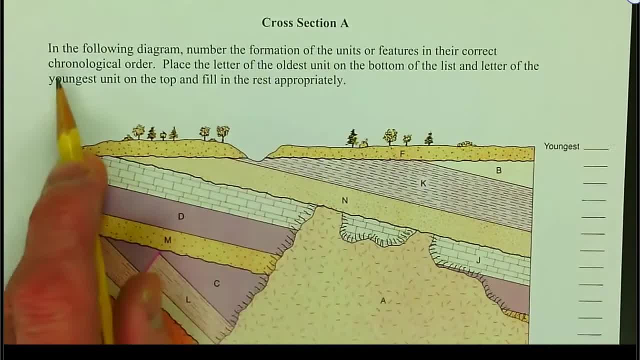 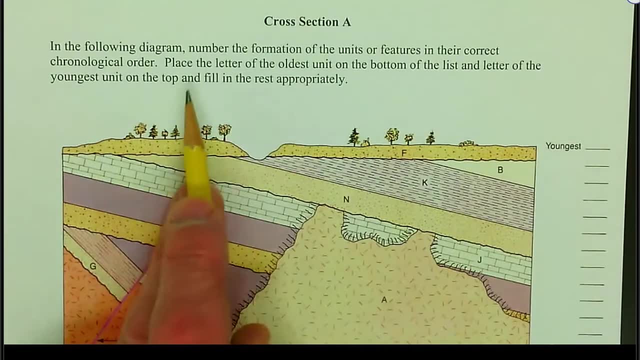 Let's take a look at cross section A In the following diagram. number the formation of the units or features in their correct chronological order. Place the letter of the oldest unit on the board of India When moon is the longest- the bottom of the list, and the letter of the youngest unit on the top, and fill in the rest appropriately. 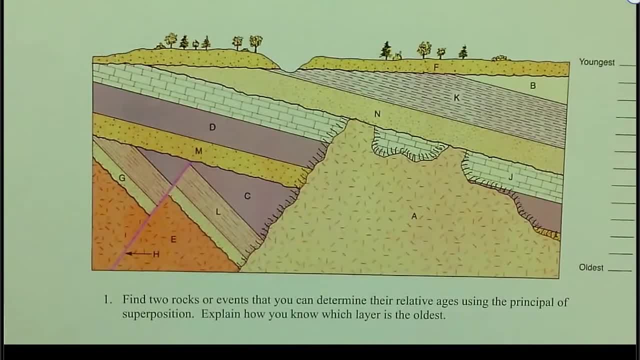 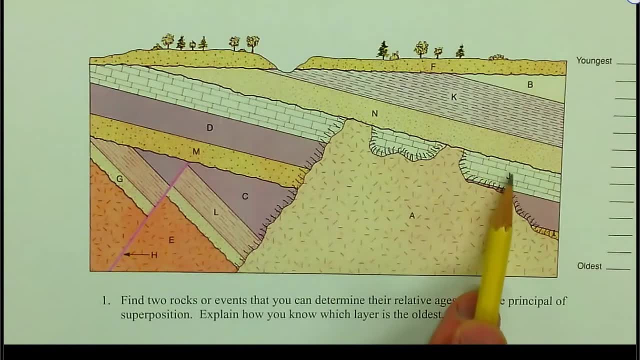 All right, let's take a look. Before we start thinking about what's older and what's younger, let's simply look at what we have. I definitely see some sedimentary rock layers, such as this layer here, which is a limestone called J. Here's a shale called K. We have a layer B and N as well. 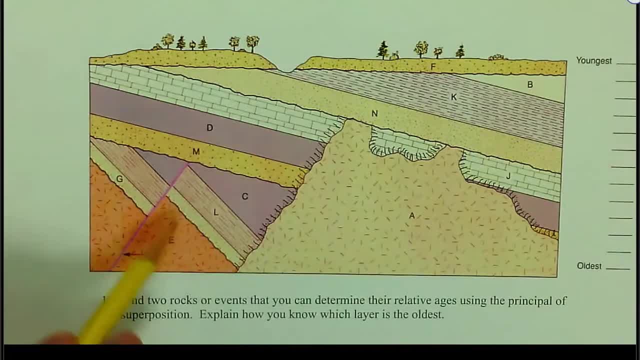 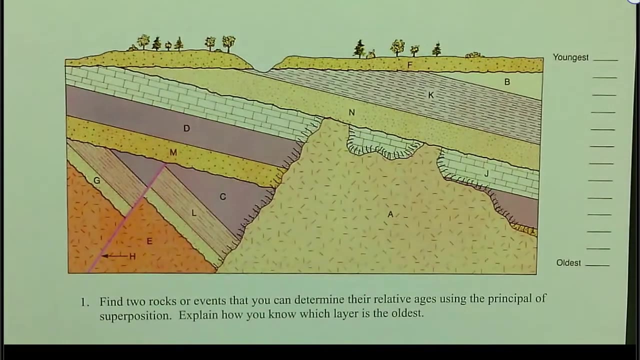 in there, D and M, some other sedimentary layers that are tilted even more. There's an igneous intrusion A, and there's also a fault that's labeled H. Almost everything in this diagram in this cross-section has been tilted some more than once, except for one young layer. 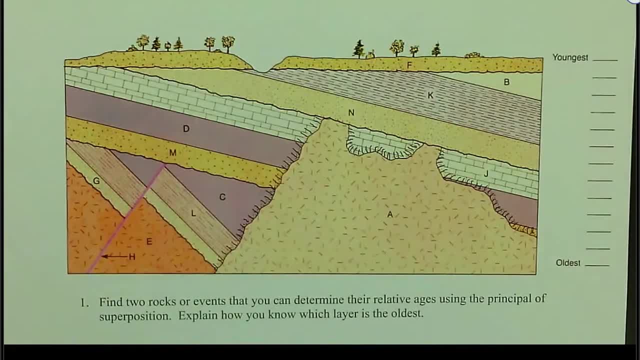 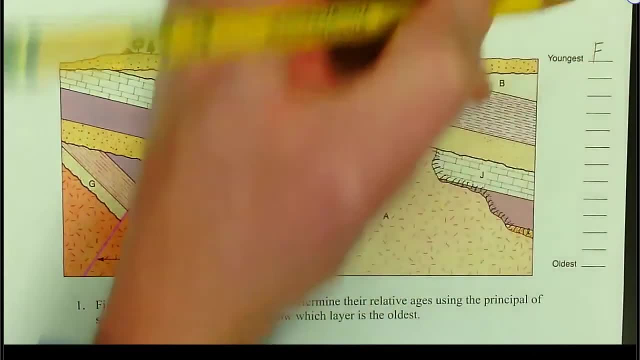 and that's layer F at the top. Notice, F has not been tilted and F is also at the top. That's going to be our youngest layer Down here at the bottom. I got this igneous intrusion A lot of times. we just automatically go: oh, if it's at the bottom. 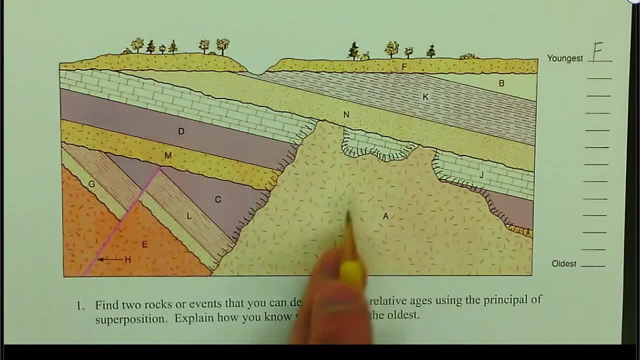 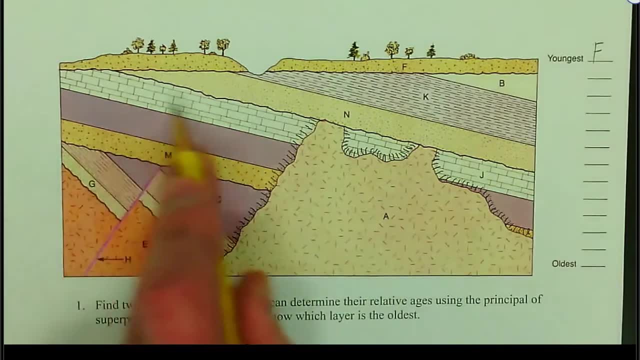 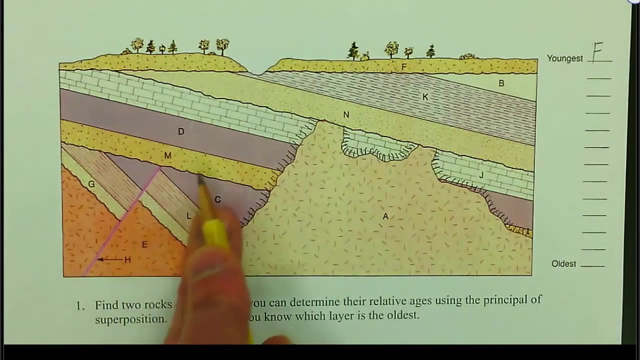 it's got to be older. but that's true for sedimentary rocks but not true for igneous intrusions. Notice that A has contact metamorphism in all of these layers over here. All of these layers have some contact metamorphism. so I can't have A happen right away. I need to get all of 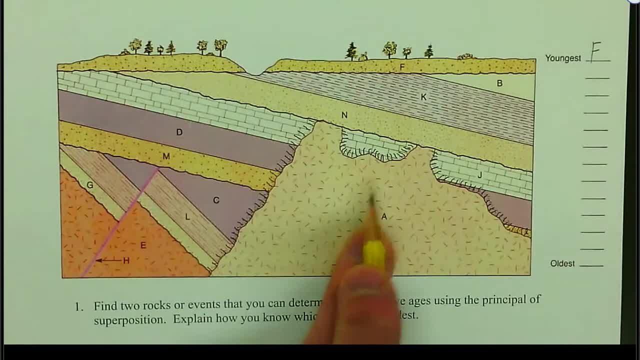 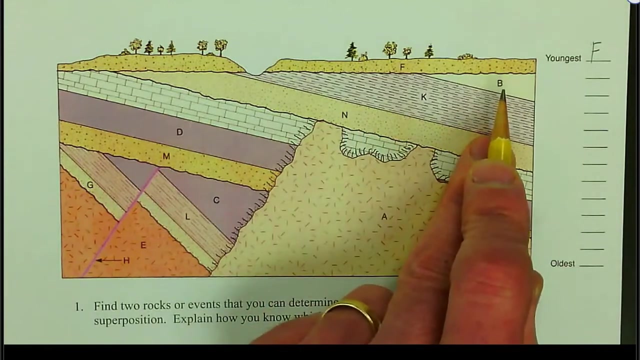 these layers first, then A, A igneous intrusion. A does not have any contact metamorphism with N. A does not intrude into N. N must come after or is younger than A. I'm going to have my oldest layers will be these. then I get A and then, after A, is N, K and B, N, K and B, with B being the. 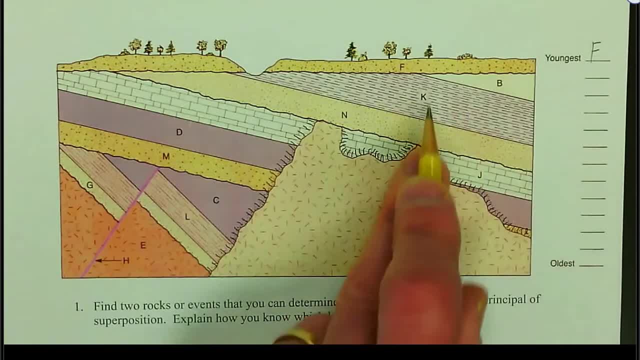 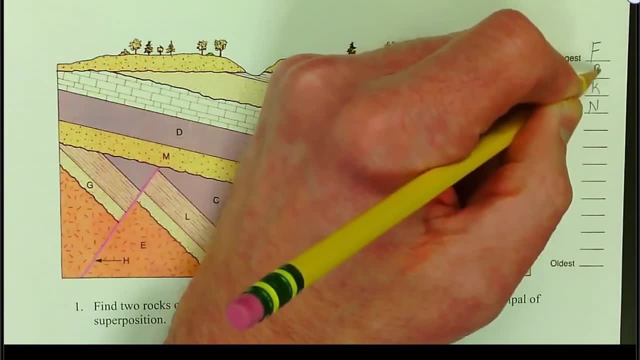 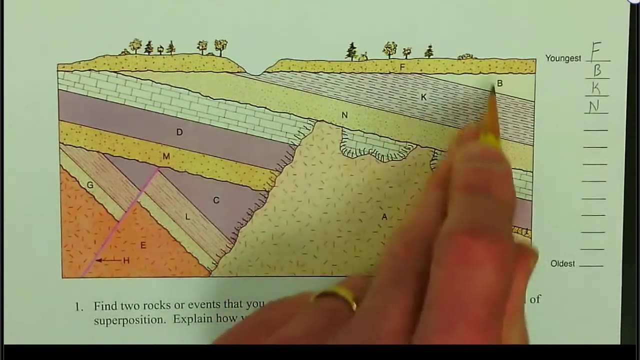 youngest of these three because it's on the top. K is younger than N because it's on the top of N. I can put N, K and B, B there, and then I have igneous intrusion. A- A does not burn those, so A must have come before. 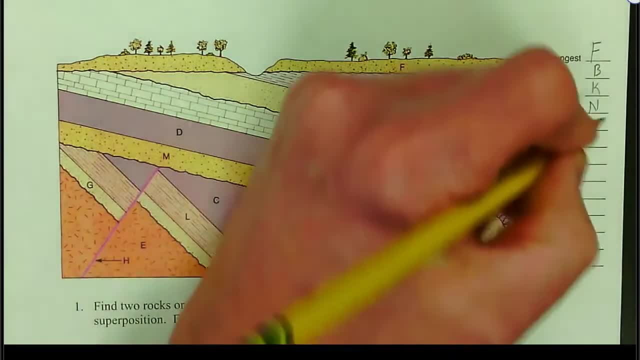 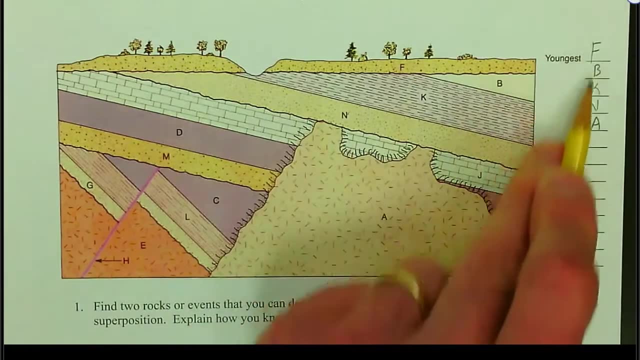 that, but it burns everything else, so it's got to be younger than everything else. The only things that A does not burn: it does not burn N K, B or F. so N K, B and F must be younger than A. 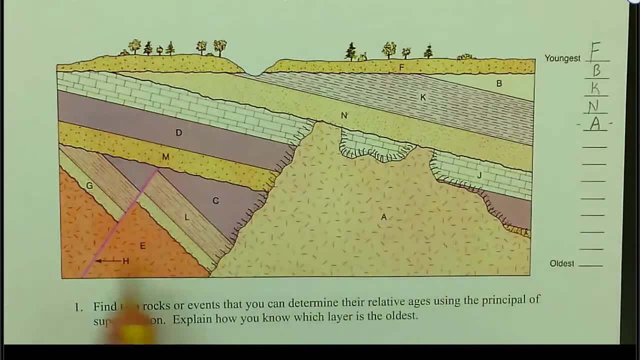 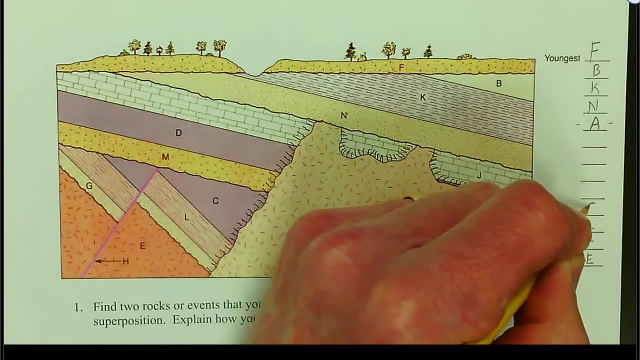 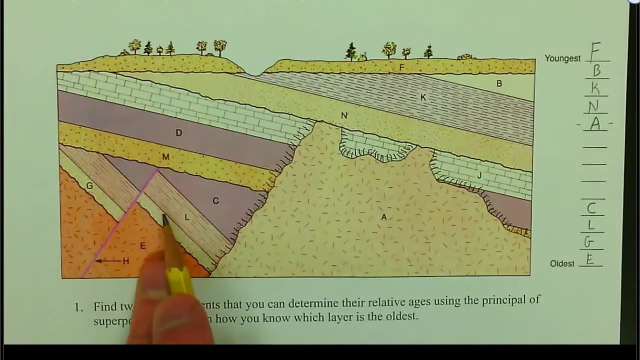 There's my igneous intrusion. A. All right, let's see if we can get what's going on over here. I've got E, G, L and C. E, G, L and C are the oldest. Then they were tilted. We have this fault H. The fault cuts through E, cuts G, cuts L and cuts C. 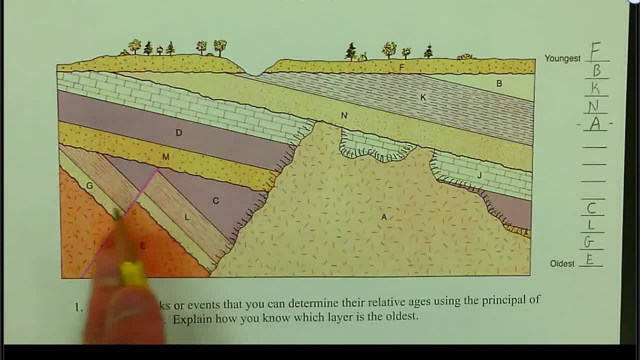 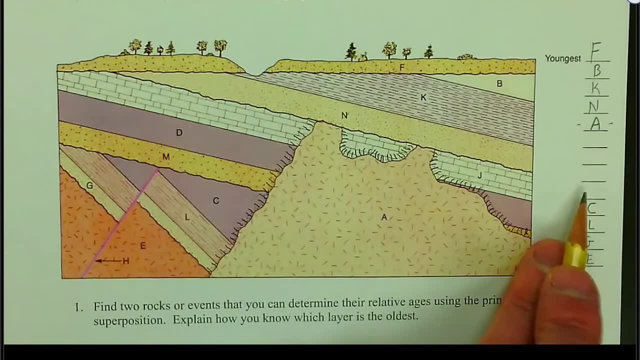 but it doesn't cut M. so that means the fault has to come after E, G, L and C, but the fault was before M. so I better make sure before I get M in here, that I get this fault H. It's got to be. 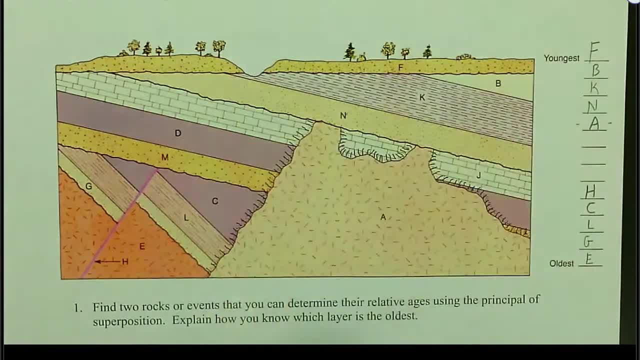 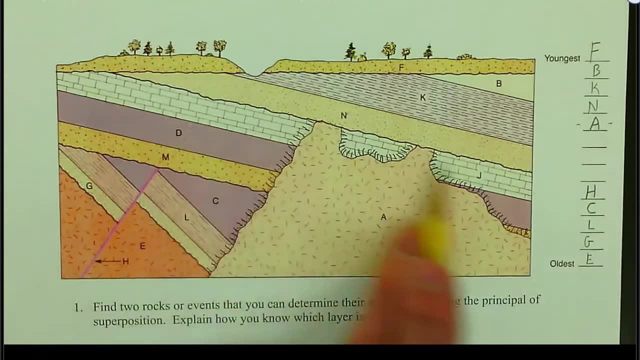 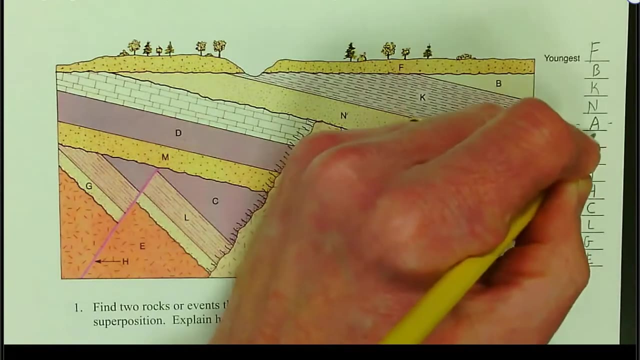 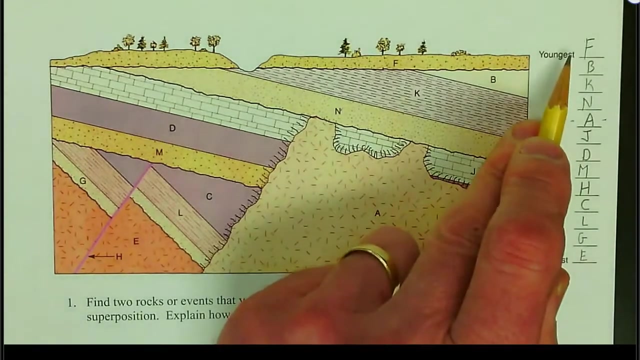 E, G, L and C. Now I've got one, two, three left for M, D and J, and we know that between M, D and J, M is going to be the oldest, J will be the youngest. Here we have the sequence of events and formation of 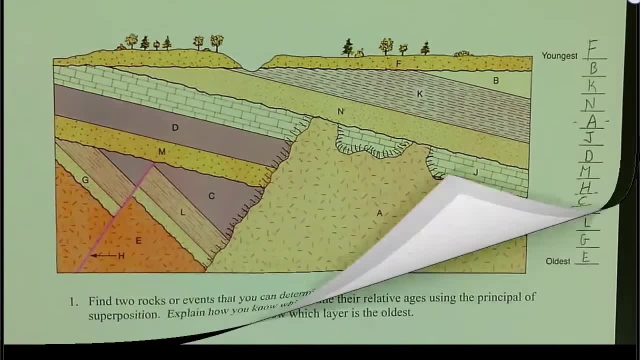 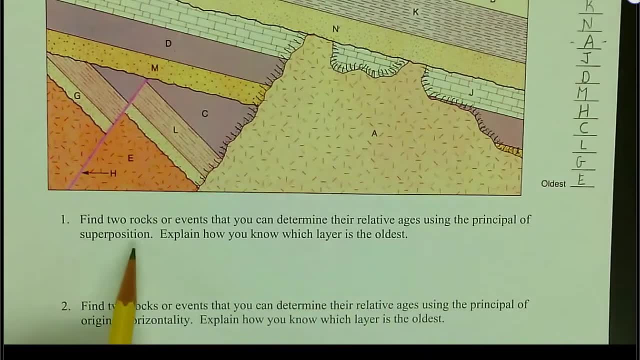 layers that formed this geologic cross-section. Number one says: find two rocks or events that you can determine their relative ages using the principle of superposition. Superposition let us know that older rocks are on the bottom and younger rocks are on the top. We have a number of different options here. I'm just going to use 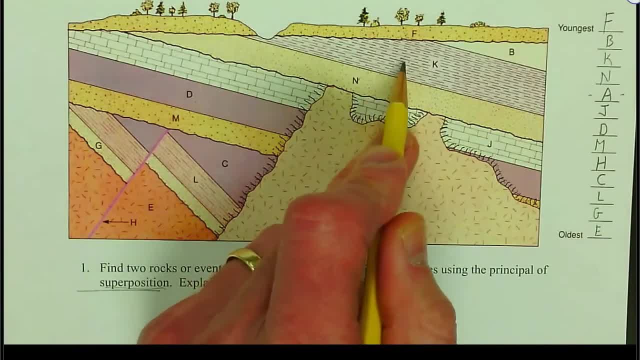 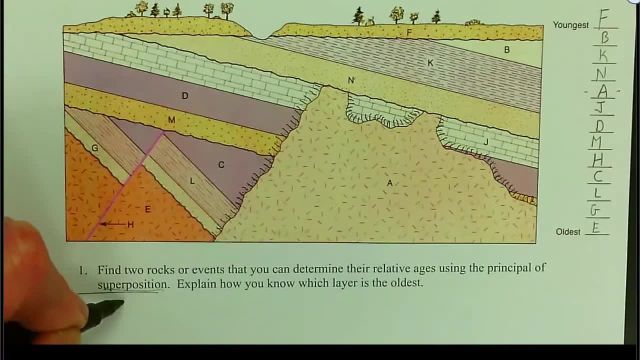 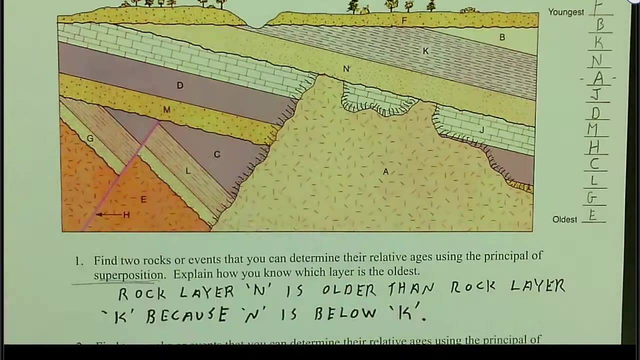 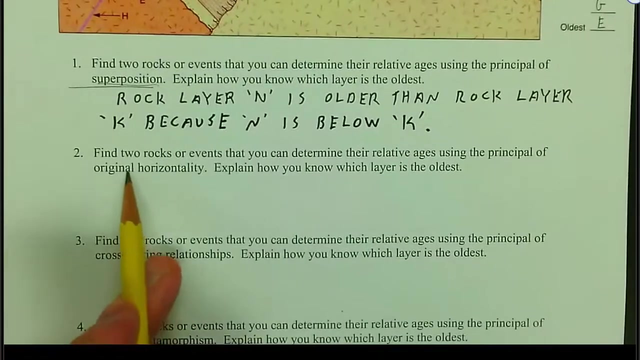 N and K. I know N is older than K. N has got to be older than K because N is below K. The next question says: find two rocks or events that you can determine their relative ages using the principle of original horizontality. How do I know the one thing is older or another, based on 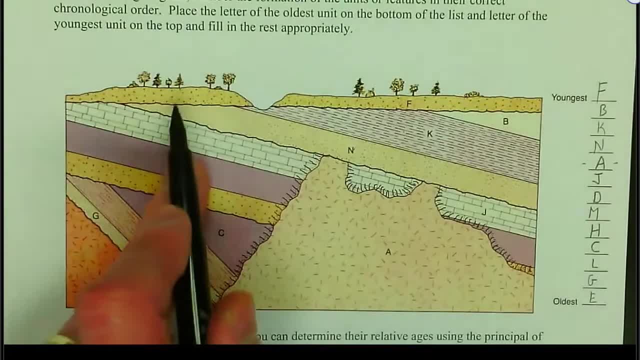 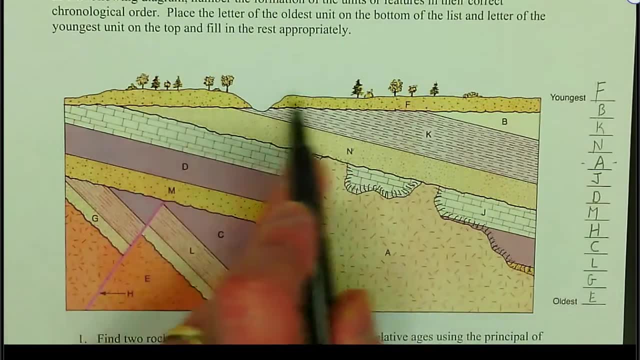 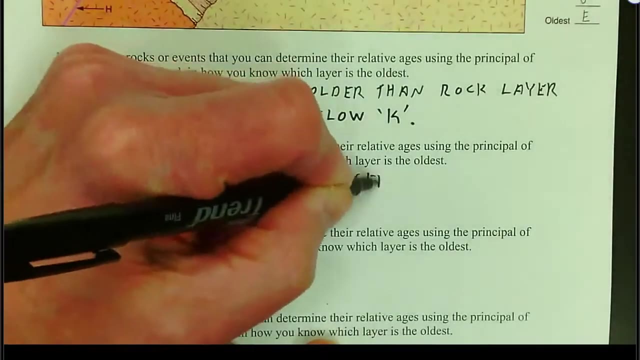 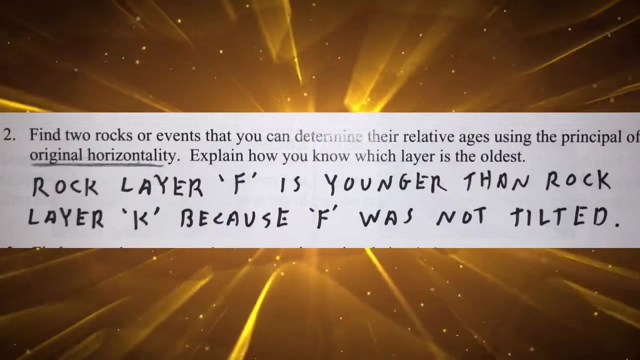 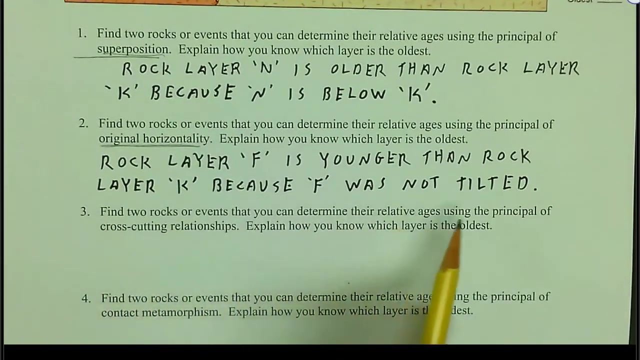 the fact that rocks are deposited horizontally. I think the best one to use here is: I know that F is younger than K Because F was not tilted and K was. Our third question says: find two rocks or events that you can determine their relative ages using. 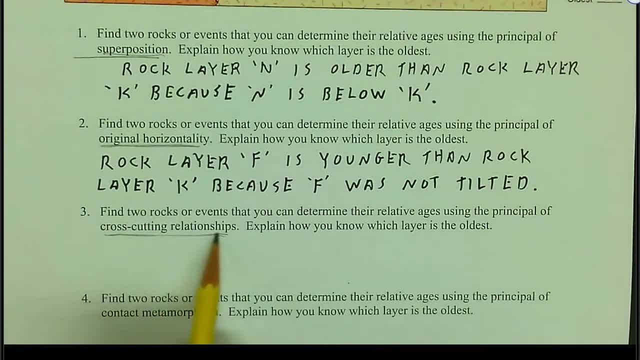 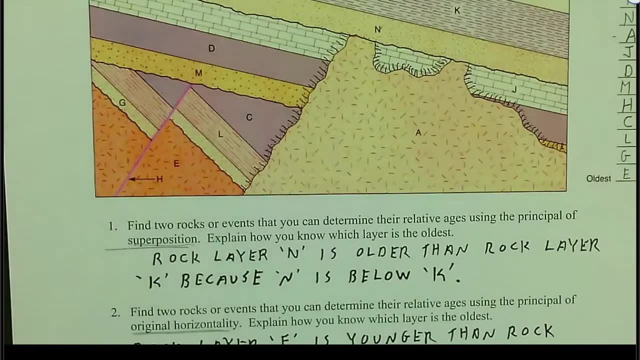 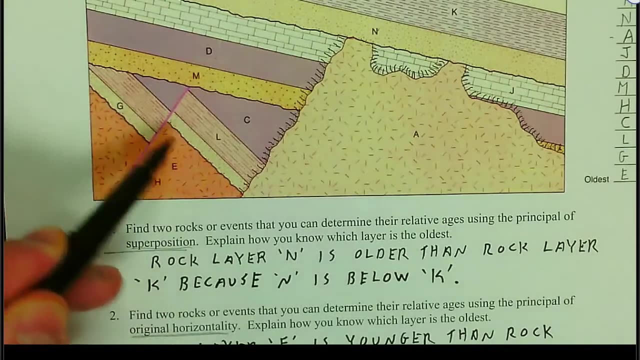 the principle of cross-cutting relationships. We want to find something that gets cut by something else. fault here We have fault H and we see that H cuts through this layer L. So there's layer L, which is the shell here, as well as the shell here. Since H cuts L, L must be older than the fault H. 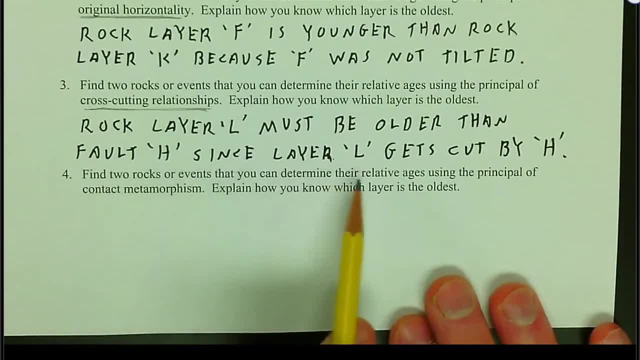 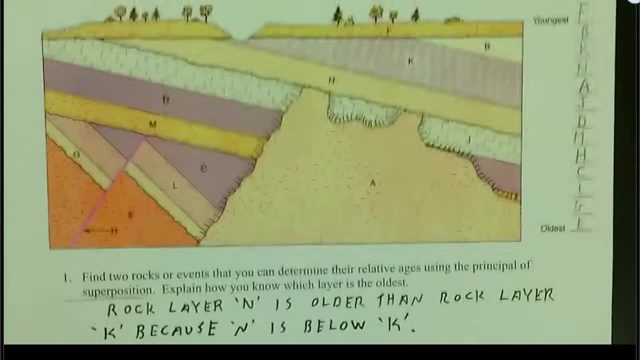 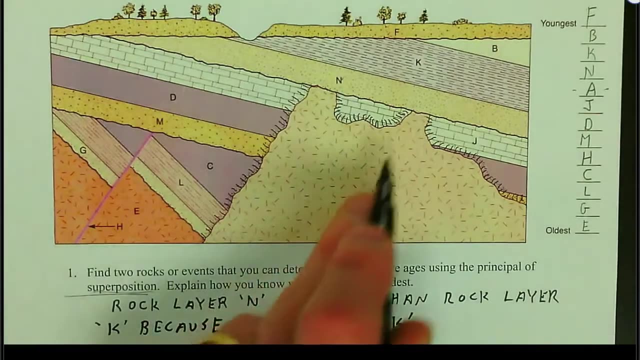 And finally find two rocks or events that you can determine their relative ages using the principle of contact metamorphism. So here we are. What about contact metamorphism? And we have some contact metamorphism with A and a whole number of rock layers For us. I know that J is older than A.